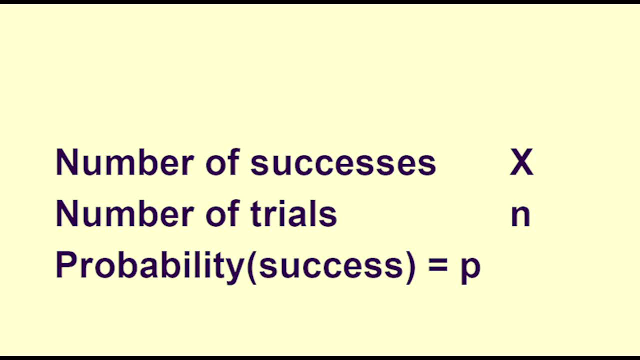 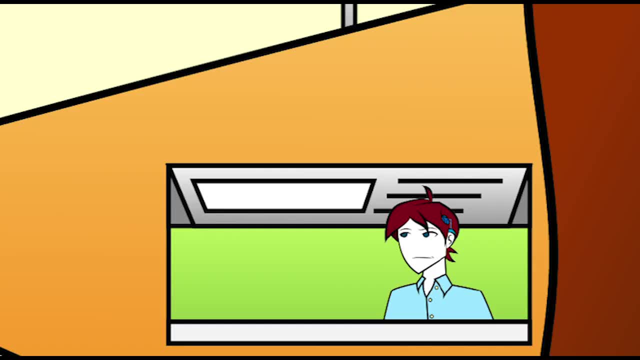 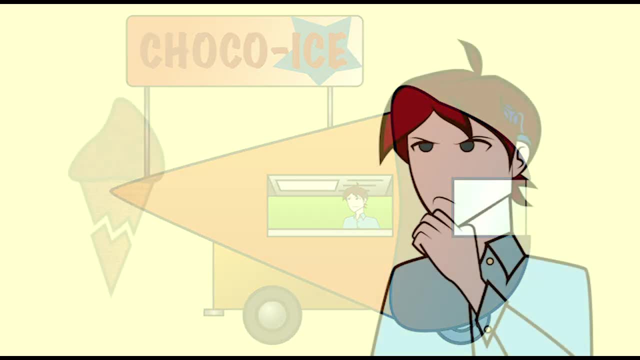 same probability, p. We state the distribution as binomial: n equals, p equals. Here is an example. Luke sells ice creams in his ice cream stand. He is concerned that his new supply of cones is substandard. Too many of them are breaking From his previous supply. he estimates that about 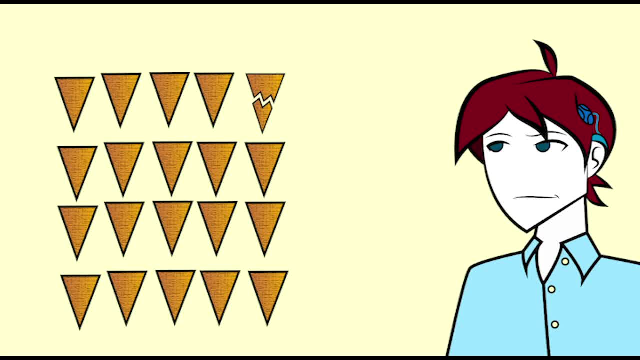 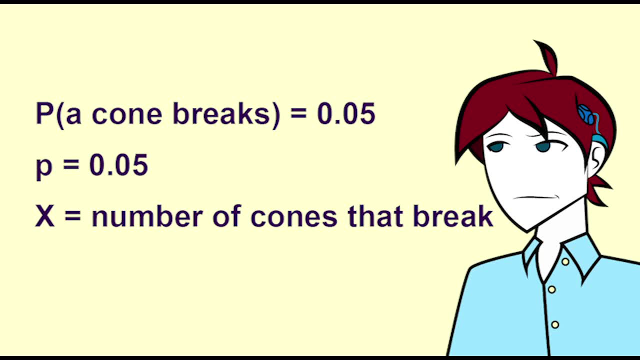 5% of cones break. This can be expressed as a probability of 0.05.. We define x as being the number of cones that break. in a box of 12 cones, Each cone has a probability of 0.05 of breaking. 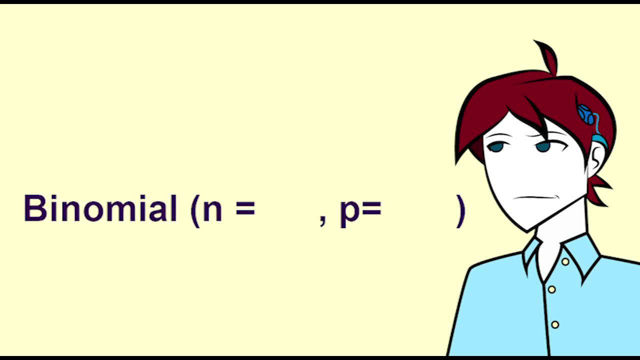 We can model this as a binomial distribution, where n- the number of trials- equals 12, and p- the probability of success equals 0.05.. In this case, we have defined success as a cone breaking. In statistics, words can mean something different from their everyday meaning. Luke wants. 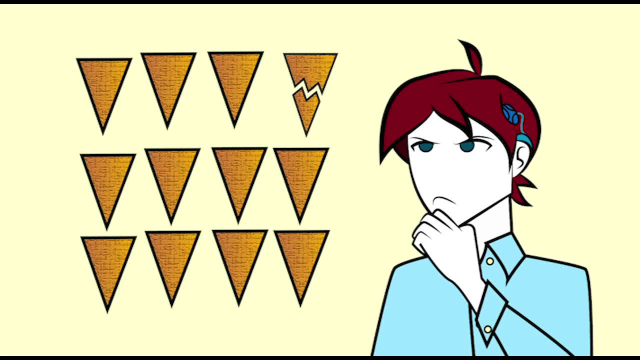 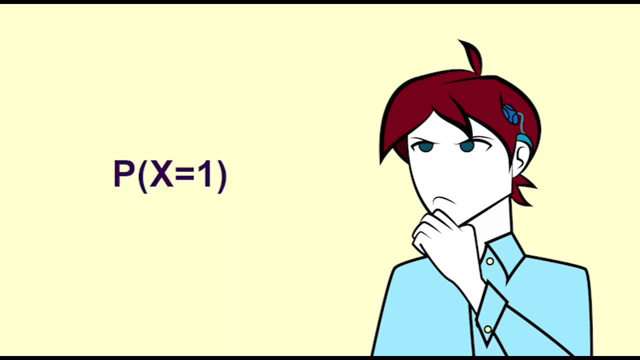 to know the probability that exactly one cone breaks out of a packet of 12.. He wants to find the probability that exactly one cone breaks out of a packet of 12.. He wants to find the probability that x equals 1.. We can use a formula, a table, a spreadsheet, an app or a calculator to find the. 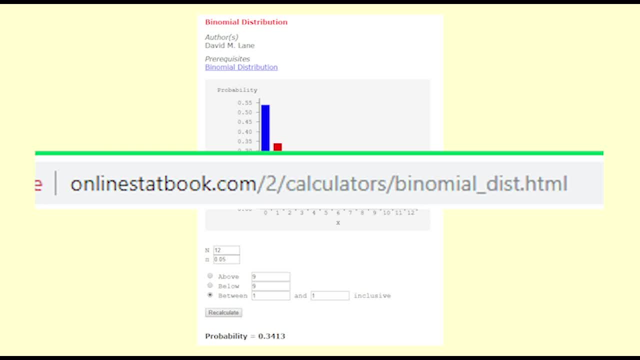 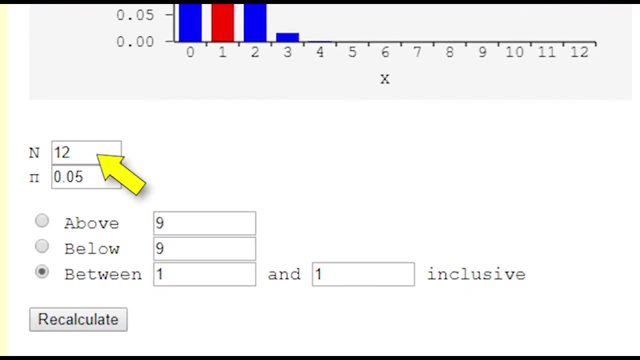 probability. I particularly like this free app found at onlinestatbookcom. I enter n of 12, the number of cones in the box and a pi of 0.05.. Sometimes the individual probability of success uses the Greek letter pi. I state that I would like to find out the probability of x, the number of 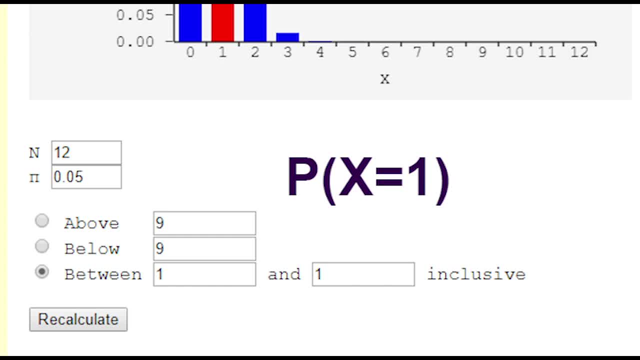 cones in the box and the pi of 0.05.. I state that I would like to find out the probability of x, the number of cones in the box and the pi of 0.05.. I do this by saying that the probability I'm 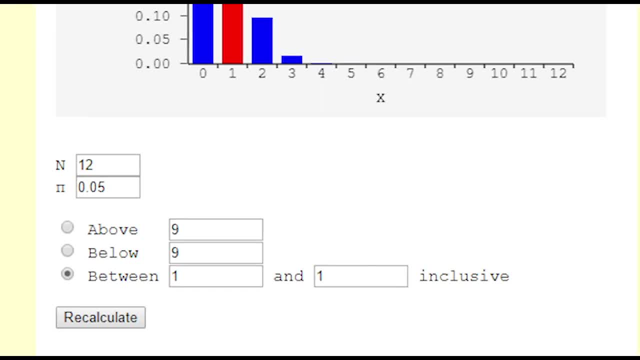 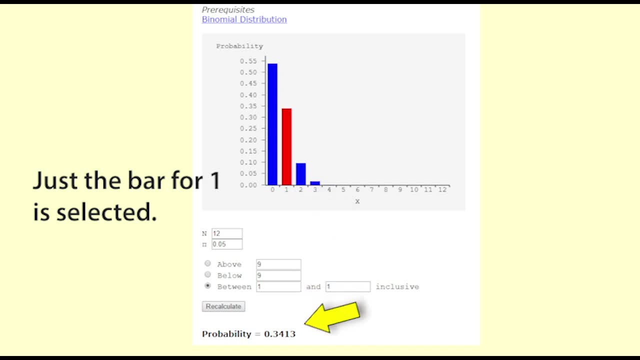 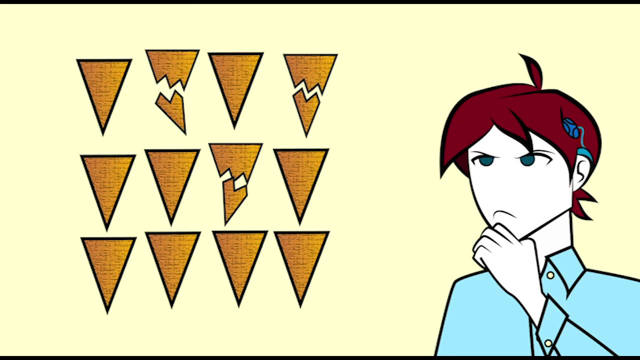 interested in is between 1 and 1 inclusive. You can check on the graph that you have the probability range that you're interested in. The answer is 0.3413 and you can see it in red on the graph. Now say: I wanted to know the probability that two or more cones break in. 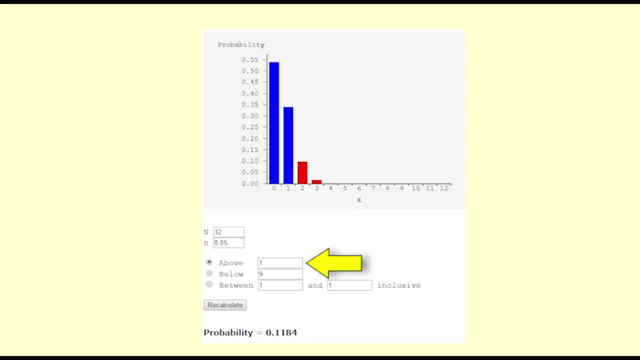 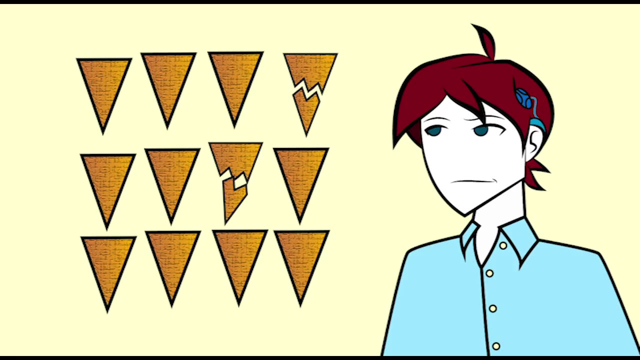 a box of 12.. I change the input to above: 1.. By looking at the graph, I can see that I've included all values 2 and above. The probability of two or more cones breaking is 0.1184.. We can use the app to explore further the likelihood of different numbers of breakages. 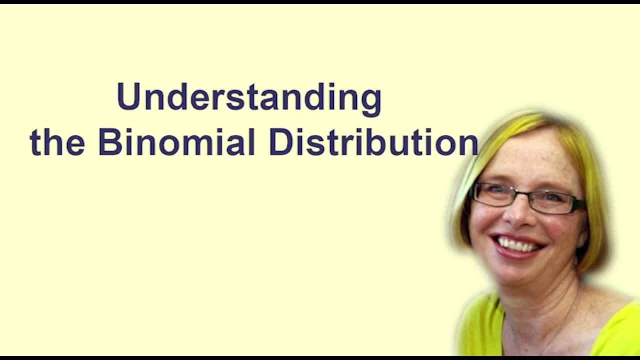 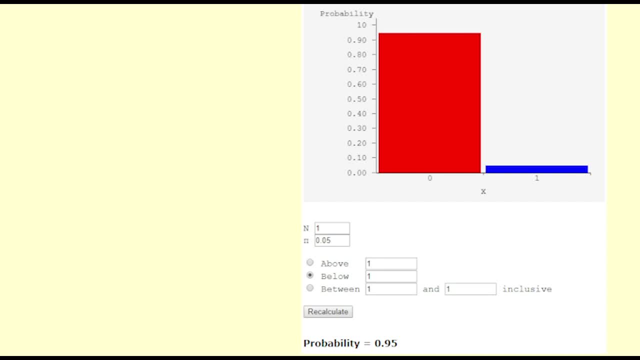 in different ranges of numbers of breakages. Understanding the binomial distribution, We will now look at where this answer comes from. Now say Luke wanted to know the distribution for one cone. It would look like this: There There are only two values that x can take. 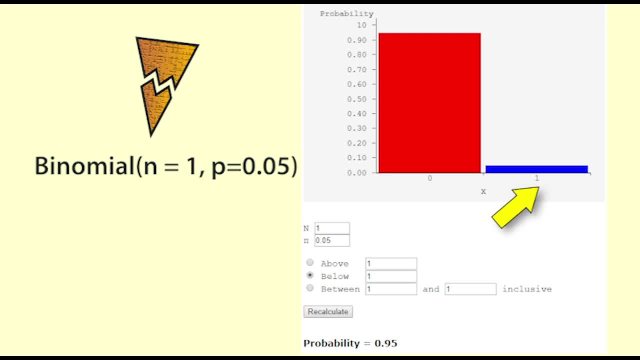 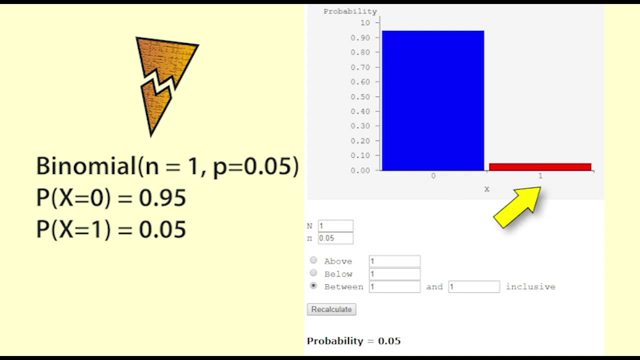 0, no breakage or 1, one breakage? There is a 95% probability that the number of breakages is 0 and a 5% probability that the number of breakages is 1.. But what about if there were two cones? 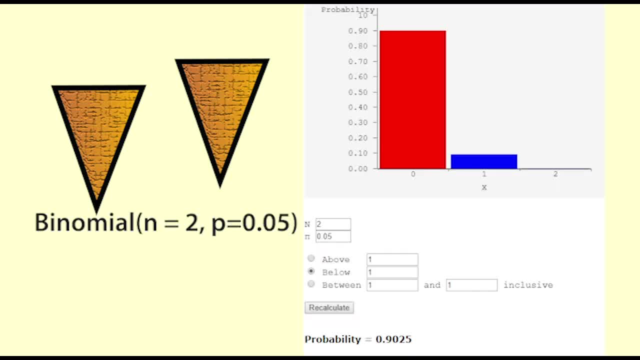 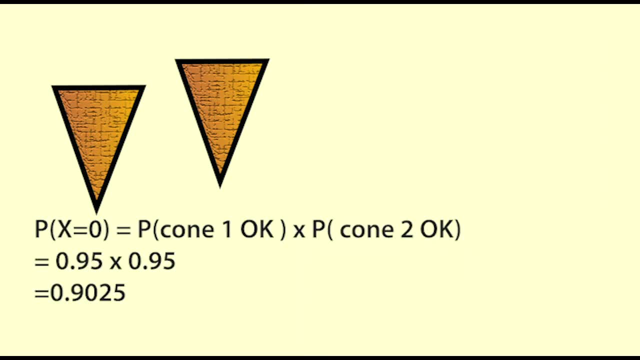 Here is the distribution for binomial: n equals 2,, p equals 0.05.. The most likely thing to happen is that no cones break. The probability for zero breakages is the probability that cone 1 doesn't break, which is 0.95,, and cone 2 doesn't break, which is also 0.95. 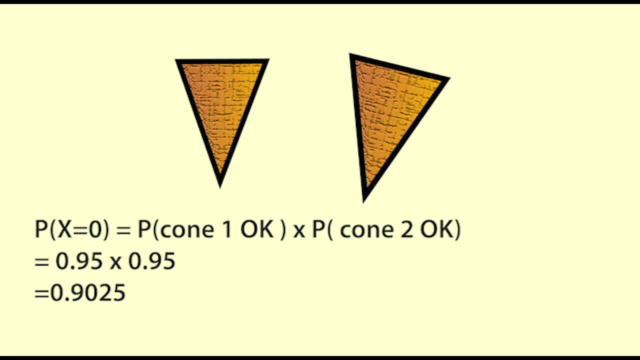 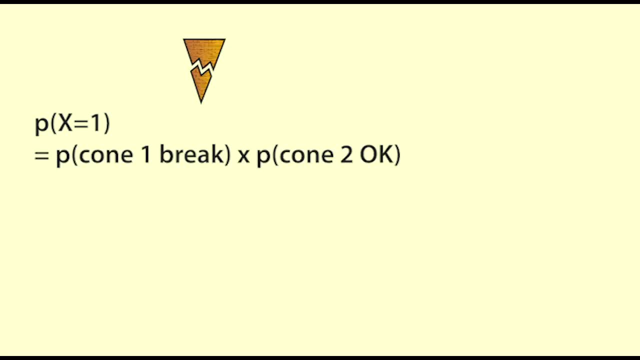 The combined probability is 0.95 times 0.95, which is 0.9025.. The probability of one of the two cones breaking is the probability of the first one breaking and the second one staying whole, or the first one staying whole and the second one breaking. 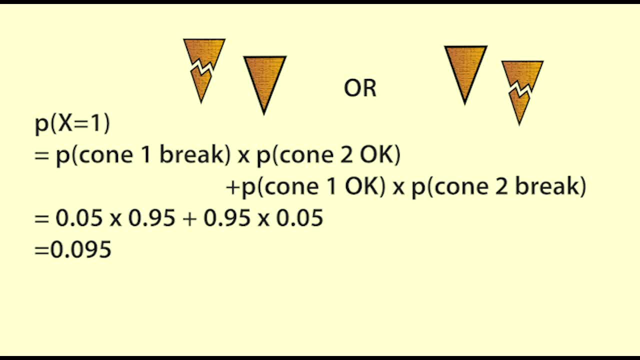 That equals 0.05 times 0.05.. 0.95 plus 0.95 times 0.05, which comes to 0.095.. Is it possible for both cones to break? Yes, but it's very unlikely. 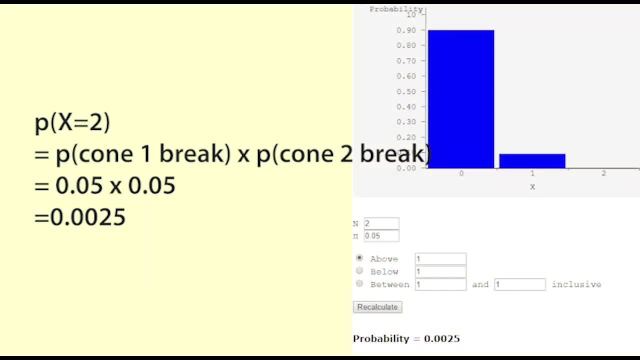 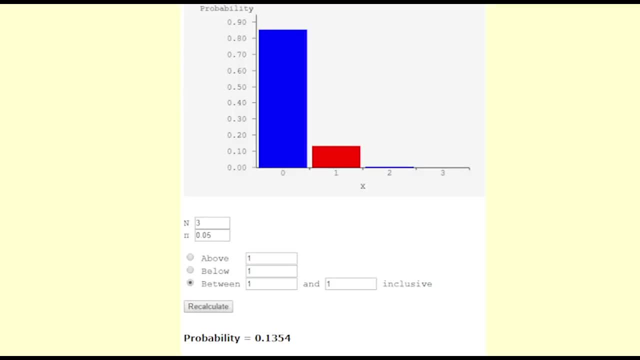 0.05 times 0.05 equals 0.0025.. And here is the distribution of breakages for three cones. As you can see, the likelihood of no breakages is getting smaller and the spread of numbers is getting greater.